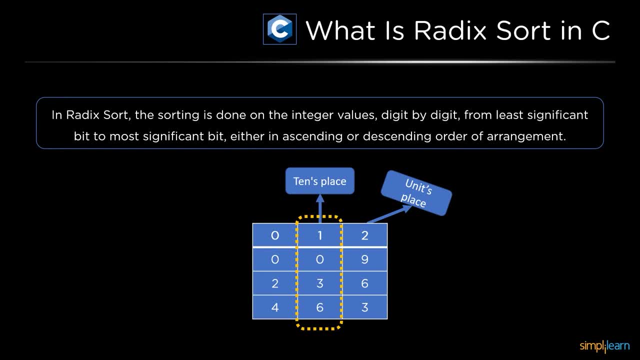 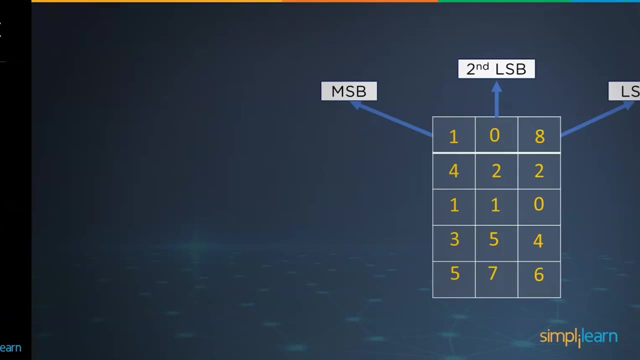 they are sorted in the proper place. move on to the tens place And sort the elements by digit, by digit, And finally sort the elements of the hundreds place. Great, Now we have an idea of what Red X sort is in C. So, moving ahead, let's understand the working of the. 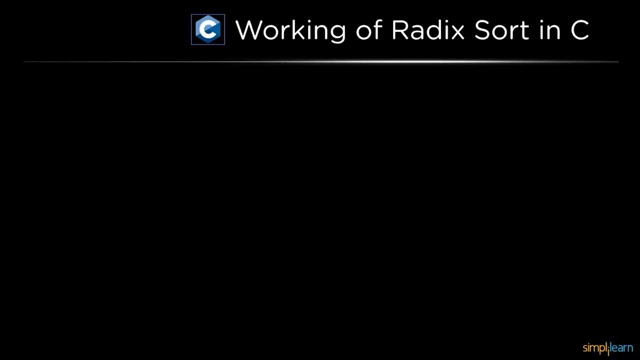 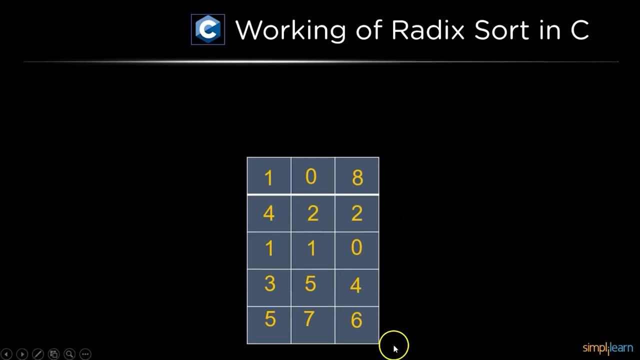 Red X sort. So let's consider this example. We have an array of five elements to sort, So first find the largest element, And it is red x, And the time constraint is 11.. So let's take an example For our game. we have to find five elements, So first find the. 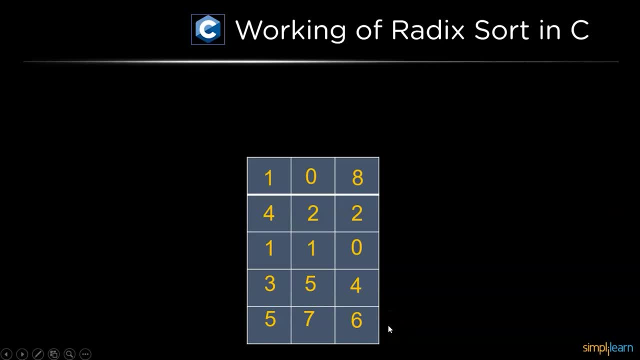 largest element, 1,, 2, and 3, and then we have five elements to sort. So let's find the 576, which consists of three digits in it. that means we required three passes to solve the unordered array. so, as i discussed before, in the first pass saw the elements starting with the. 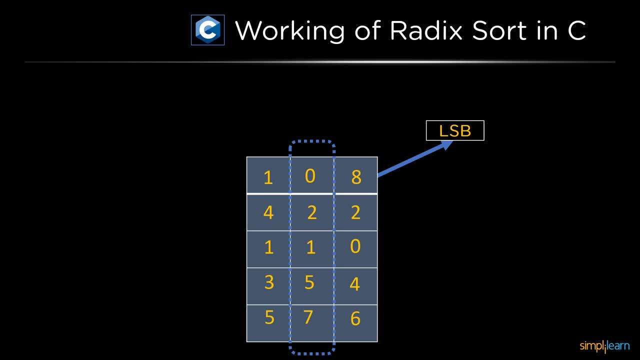 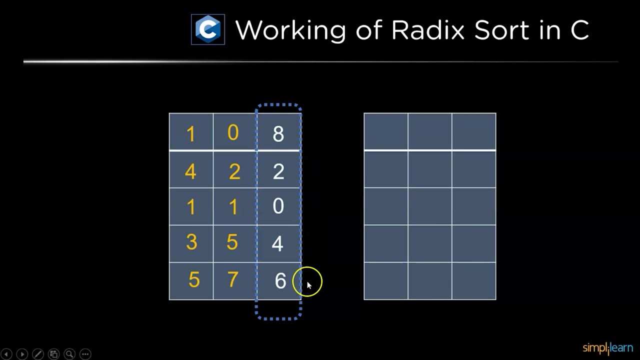 least significant bit, followed by the second least significant bit and later the most significant bit: elements. so here the least significant digits are 8, 2, 0, 4 and 6.. so, considering digits 0 to 9, we use counting sort to sort the elements and place them in the right order and at the proper position. 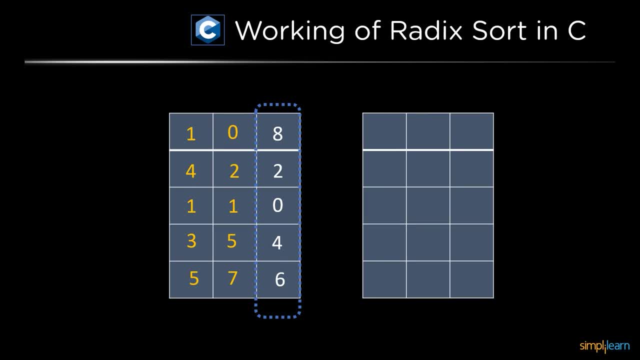 so, since we have 0 in the list, let's place this element first and then search for the next least element in lsb, and it is 2.. and, followed by 2, we have 4, and then 6, and the last element is 8. 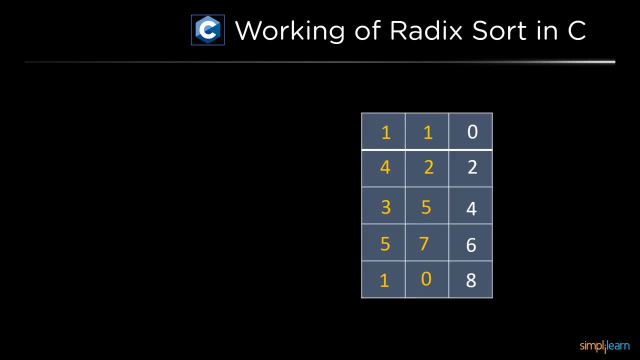 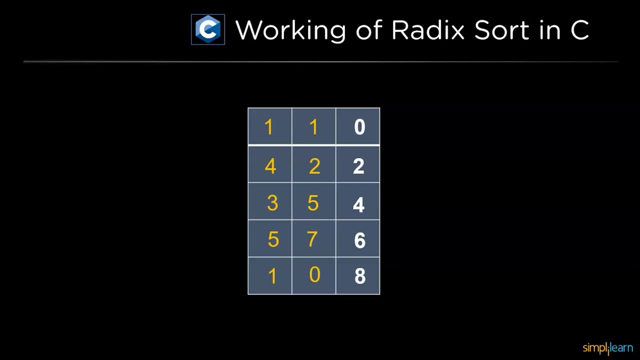 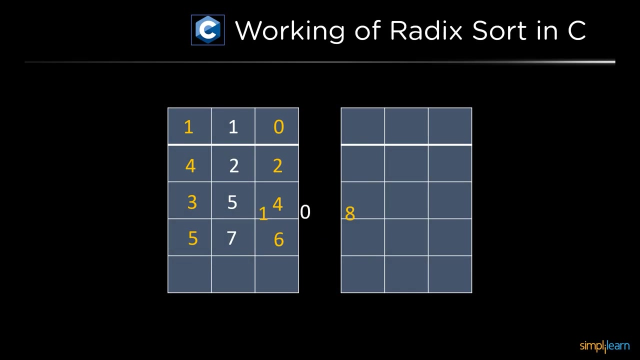 and finally, the digits are sorted, and the sorted elements are in the ascending order of 0, 2, 4, 6 and 8. so now, moving on to the second least significant bit, the elements are 1, 2, 2,, 5, 7 and 0. So the least digit we have in a list is 0. So let's place the digit first. 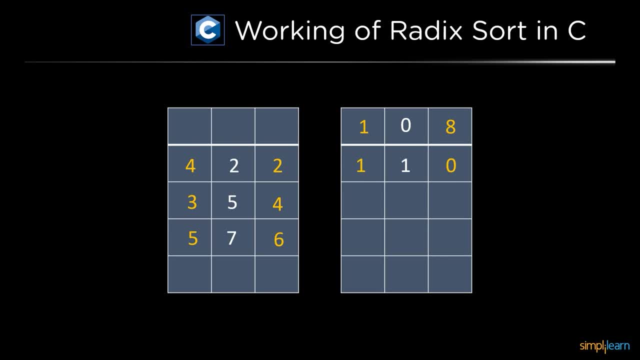 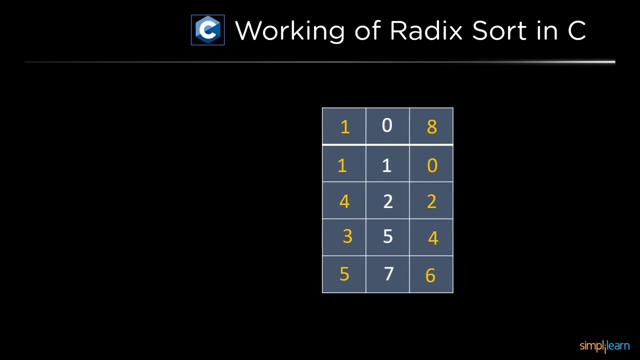 and followed by digit 0, we have 1, next Then 2, and followed by that we have 5 and 7.. So here, finally, the order of sorted elements is 0,, 1,, 2,, 5 and 7.. Similarly, let's move. 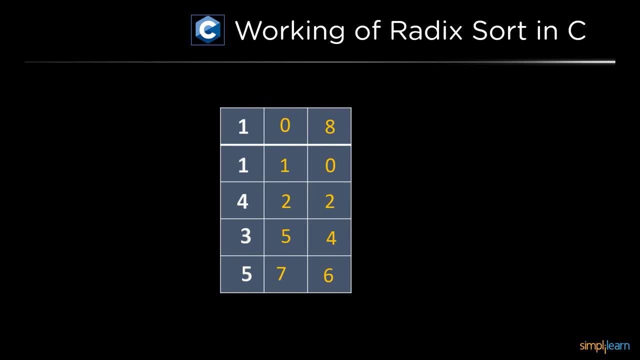 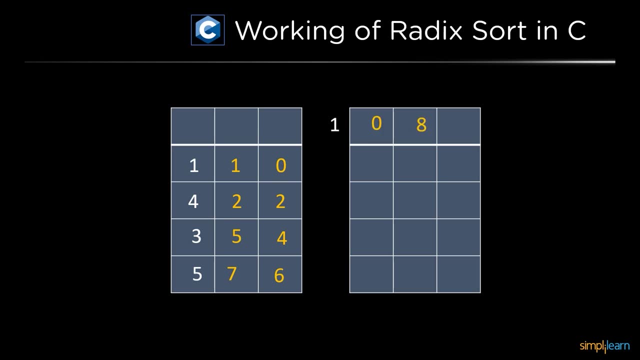 on to the most significant bit. So let's place the least digit first, which is digit 1.. So, followed by that, we have another 1. So let's move that next. Then the next least digit is 3.. Followed by 3, we have 4 and then 5.. Finally, the elements are sorted in. 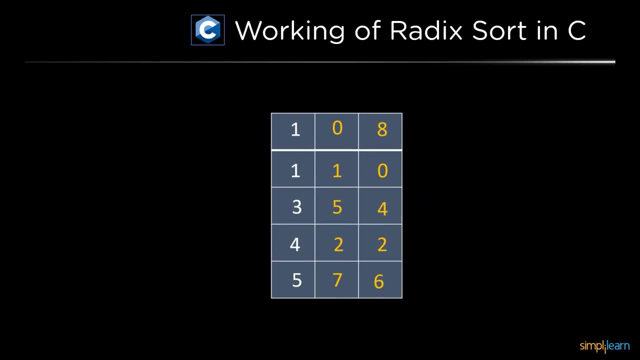 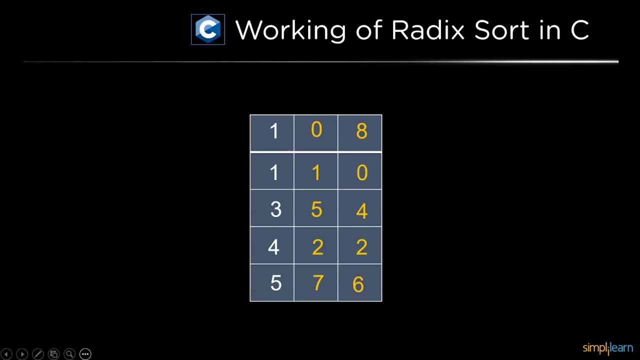 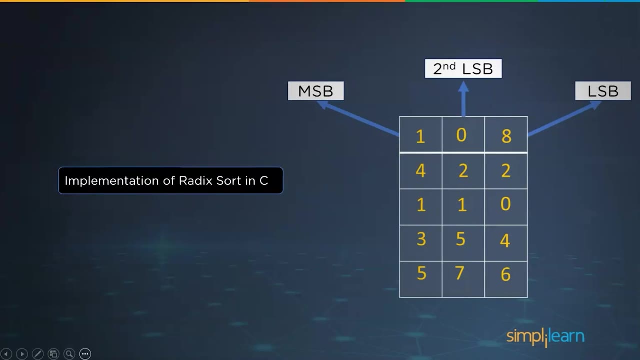 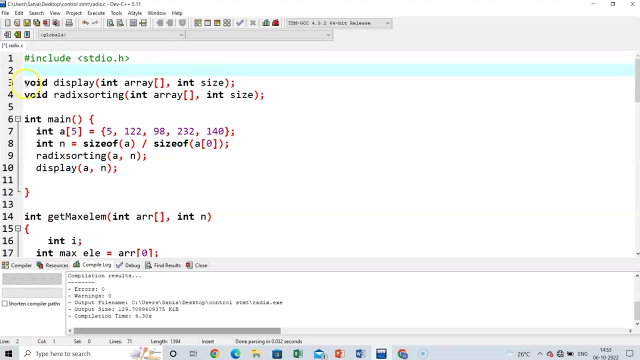 the right order. The array elements are sorted in the ascending order, and they are 108,, 110,, 354, 422 and 576.. Okay, so let us now move on to the implementation of RedXSort in C. So it is an implementation of RedXSort. So first we have the two function declaration: 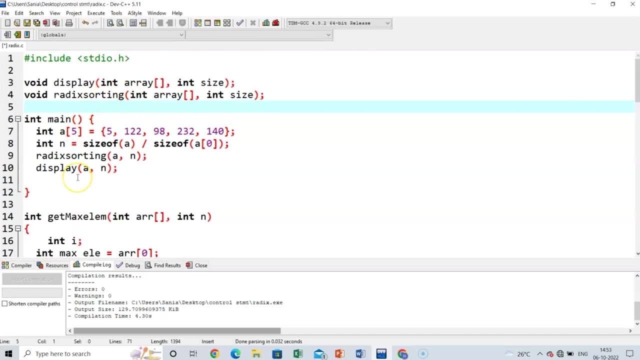 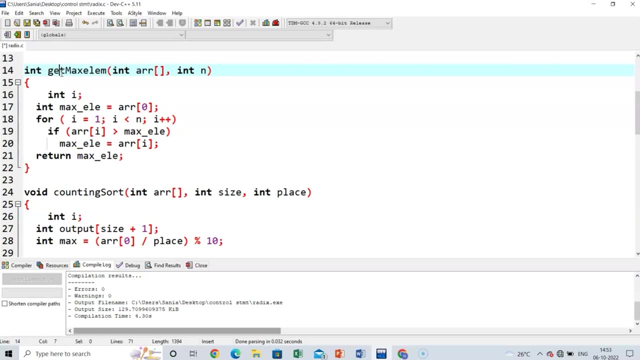 that is, display and RedXSorting. So first, moving on with the function getMaximumElement. So find the maximum number from the given array elements. So to find, we have the variable declaration maxElement. Initially a is assigned And for i is equal to 1 till i less. 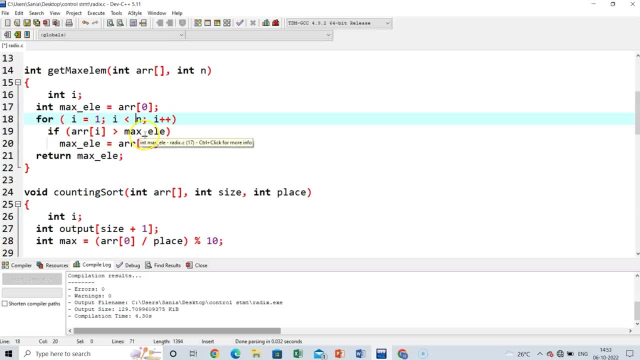 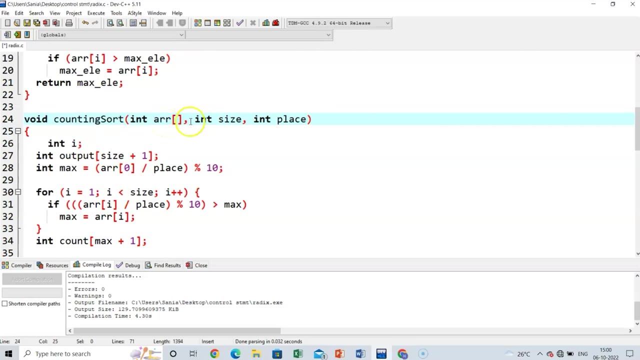 than n. If the condition a is greater than maxElement, assign e to maxElement and return max. The next function is the countingSort. So using counting sort algorithm we perform a RedXSort. So the variable declared are array, size and place. So first we are creating the output array of size plus 1. Then we are creating: 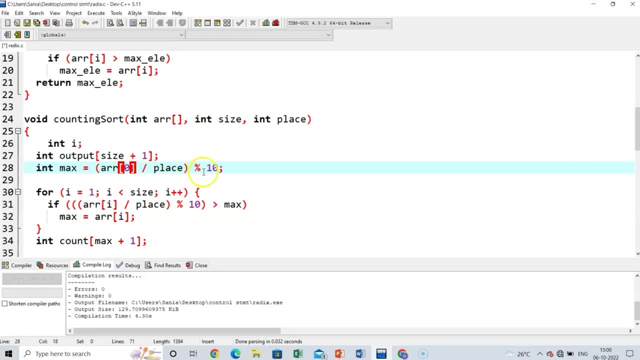 a max variable is equal to array of 0 divided by place of module 10.. And in this for loop, this for loop is to sort the array elements, So the for loop is to sort the array elements. So in this for loop, the for loop is to sort the array elements, So the for loop is to: 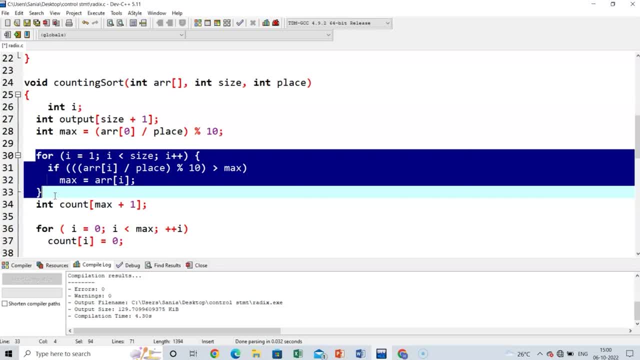 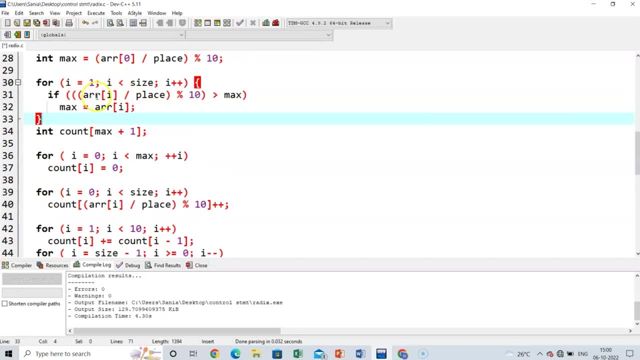 sort the array elements. So for that we are taking digit by digit, starting from unit place to 100 place. So the condition is for i is equal to 1 till i less than size. If condition array of i is divided by place of module, 10 must be greater than max. then assign: 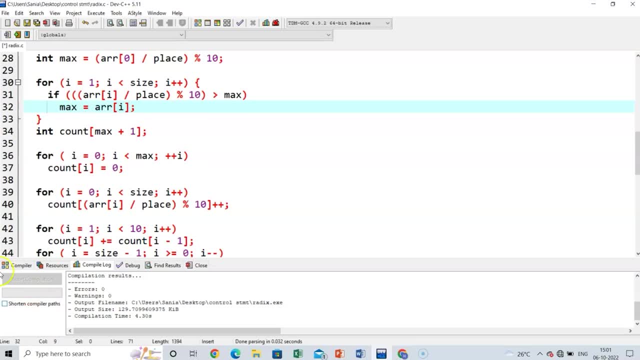 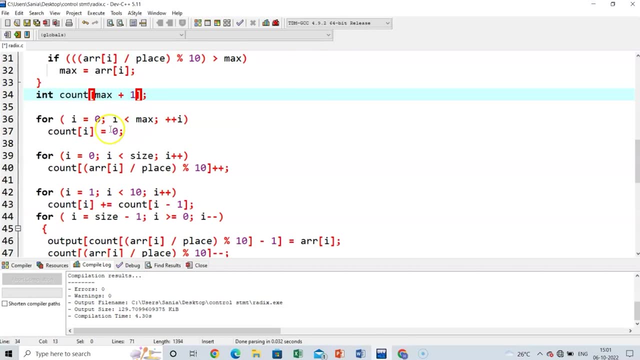